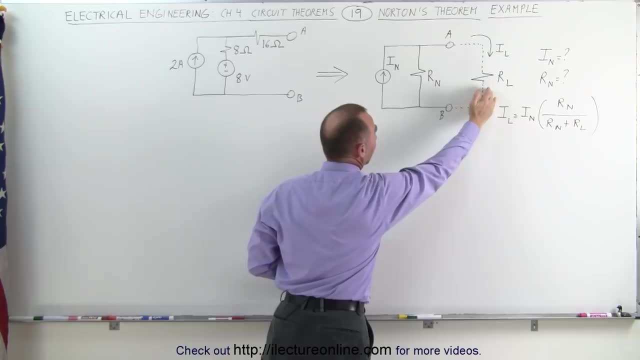 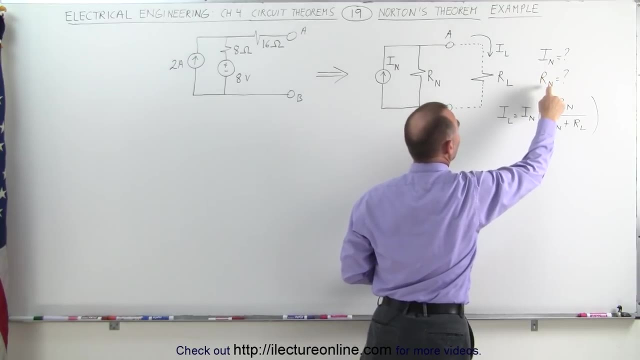 and then we have terminals A and B to which we're going to connect some low resistor. To find the current through the low resistor, we need to find the Norton's current and the Norton's resistance so that the load current is equal to this equation. right there? 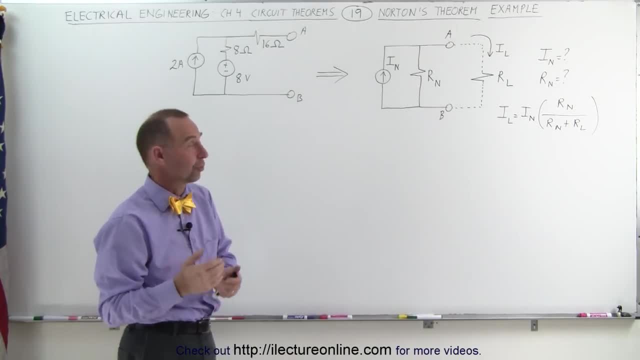 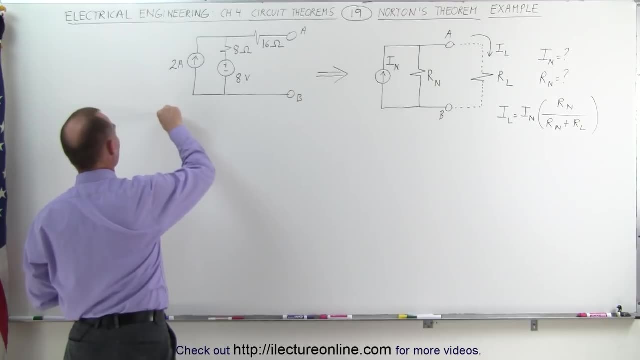 So the question is: how do we find Norton's current and Norton's resistance for the equivalent circuit? that looks like this: Well, starting out with the Norton's resistance R, sub n, it turns out that it's equal to the Thevenin's resistance. We use the exact same. 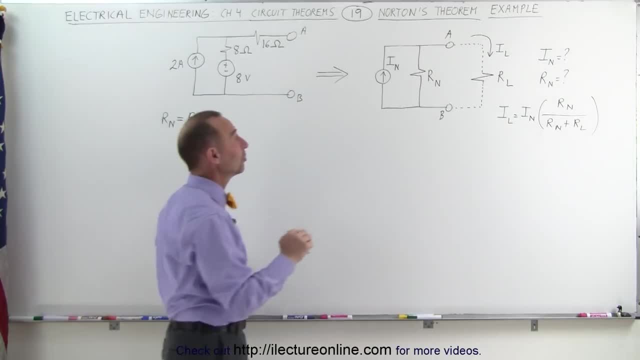 method to find the equivalent resistance. Remember that with Thevenin's resistance we had it in series with the voltage source. In this case we're going to have the Norton's resistance in P. To find the Thevenin's resistance or the Norton's resistance, we take the circuit here, we remove. 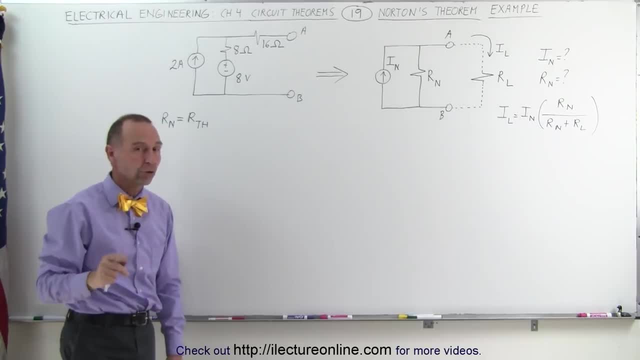 any current sources and we drop the voltage across the voltage source to zero. That means we get the following circuit. We'll have an open right here, where the current source normally goes- the 8-ohm resistance. the voltage source goes to zero, so we can just skip that and 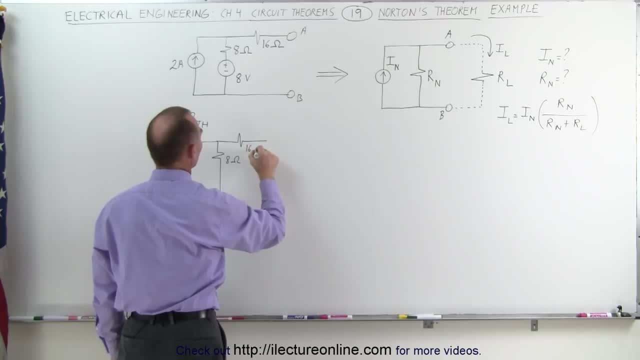 then we have the 16-ohm resistor there, 8 ohms, 16 ohms. here we have terminal A and terminal B. We leave it open and the resistance, the Norton's resistance, can be found by simply. 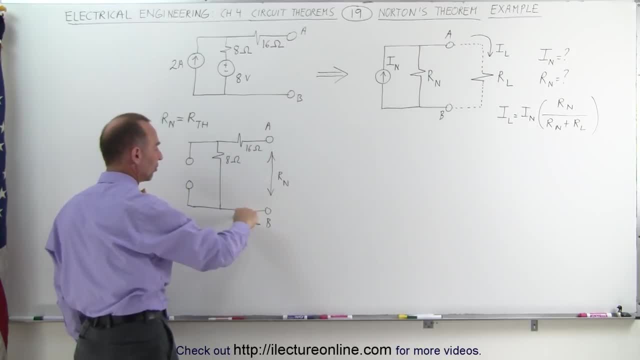 measuring the resistance between A and B, which in essence will simply be the sum of these two resistors, R sub n will be equal to 8 ohms plus 16 ohms, which is 24 ohms. Now they have the Norton's resistance. let's find the Norton's current To get that. what? 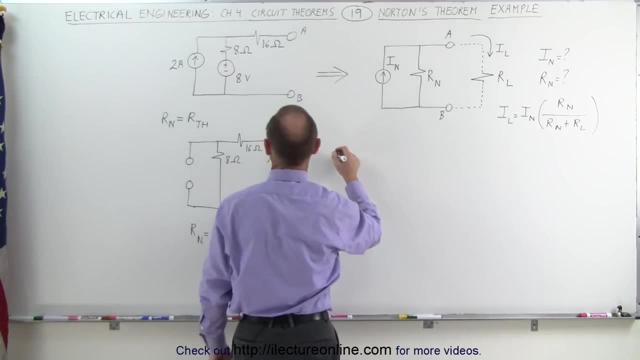 we need to do is take the original circuit, so let's redraw it. and we're going to have the Norton's resistance, So let's redraw that. Here's the 2-amp source, the 8-ohm resistor, the 12-volt- not 12-volt, it's 8-volt- voltage source. this is an 8-ohm resistor. 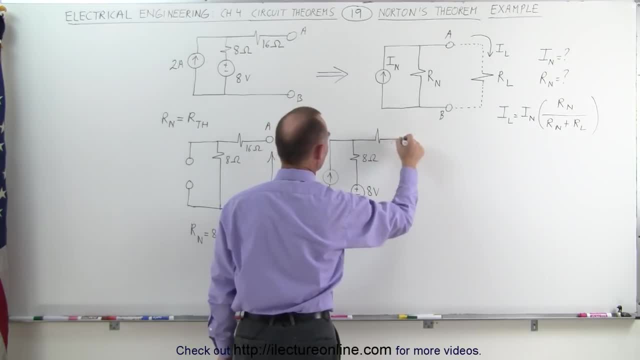 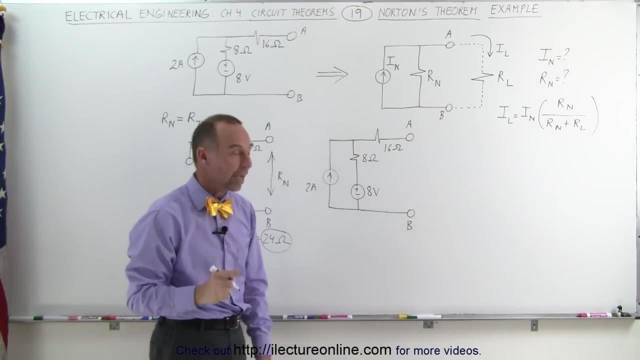 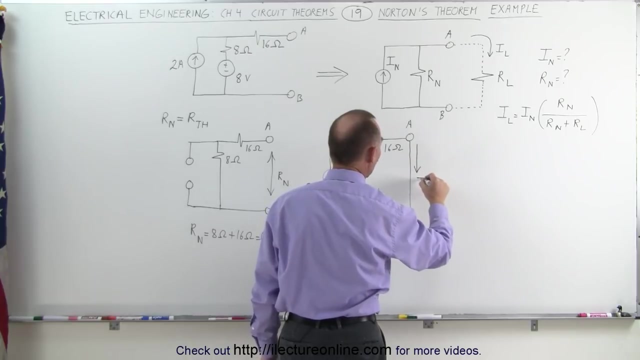 this is a 2-amp current source. we have the 16-ohm resistor here, terminal A and terminal B. To find the Norton current we have to short out the terminals A and B And then whatever current we will have between A and B that will become Norton current. How do 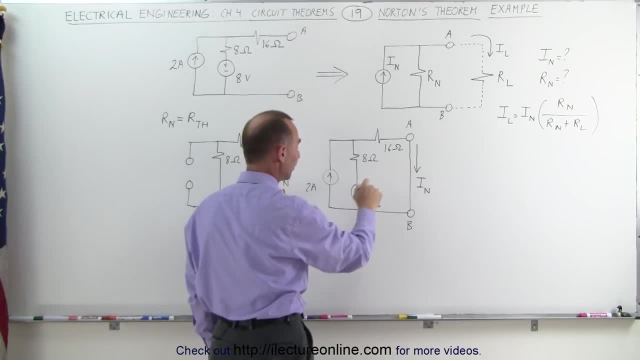 we find that. Well, simply, we're going to add up the voltages around each loop, except for the first loop. we can imagine that the current around the first loop is going to be equal to the 2-amp source. So this is I1, we can say I1 must equal 2-amps. But now we're 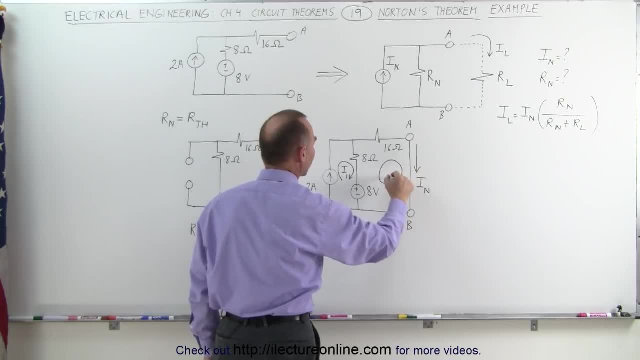 going to add up the voltages around loop 2, assuming that we have a current I2 flowing through loop 2.. A1- R is that I2 will be equal to I sub n. So all we have to do here is find I2.. We're going. 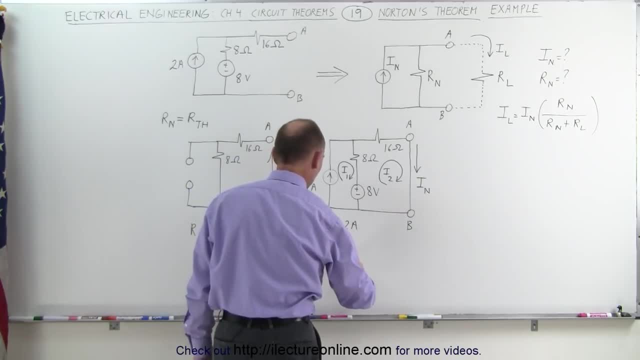 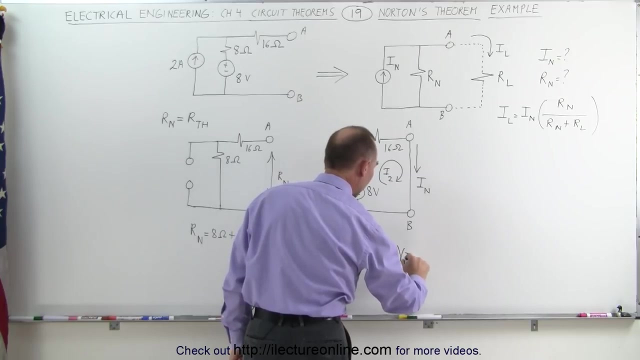 to sum up the voltages, sum up the voltages around loop 2, and that is equal to: starting from this point, that's plus 8 volts, minus the voltage drop across this resistor, which would be minus the resistance times, the current I2.. However, there's also an I1 current flowing. 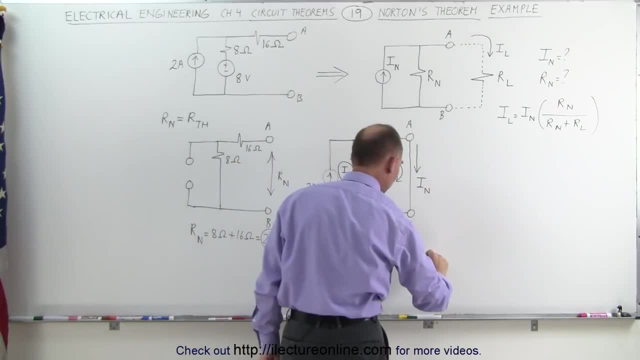 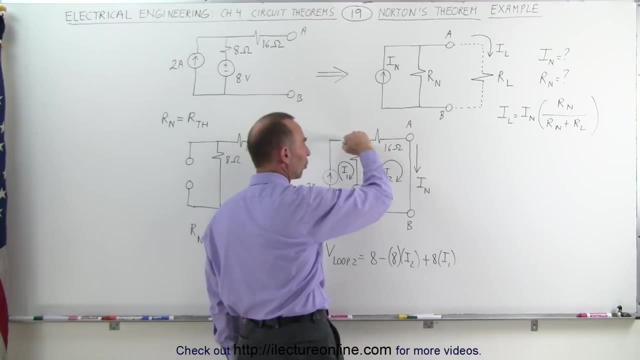 here and we're going against the current, against I1, that's the voltage rise plus 8 ohms times I1. Then, going around the corner, we go across this resistor, that's with the current I2, therefore, that's the voltage drop minus 16 times I2.. And then we go all. 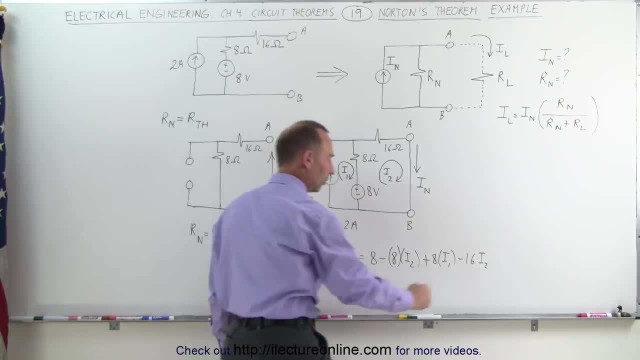 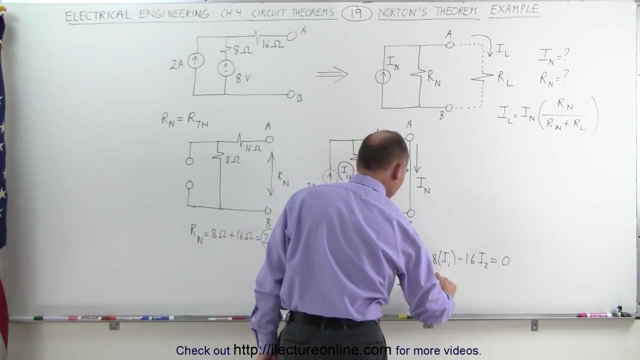 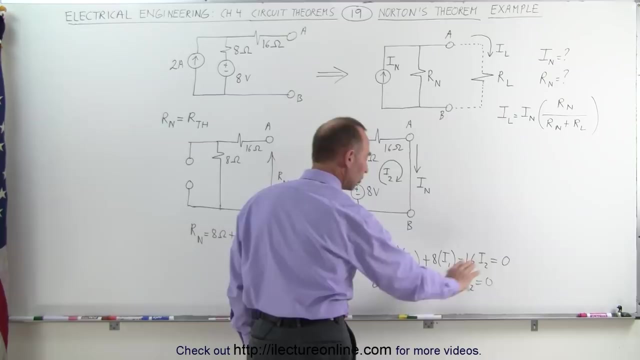 the way around, get back to where we started. that adds up to 0.. Now, knowing that I1 is equal to 2 amps, I can replace this by 2, so we get 8 minus 8 I2, plus 8 times I1, which is 2 amps minus 16 I2, equals 0.. Moving all my I2s to the 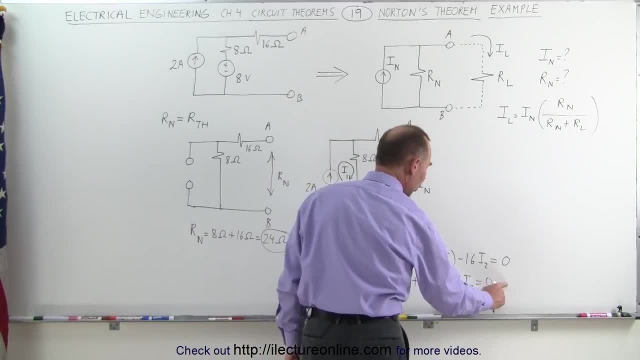 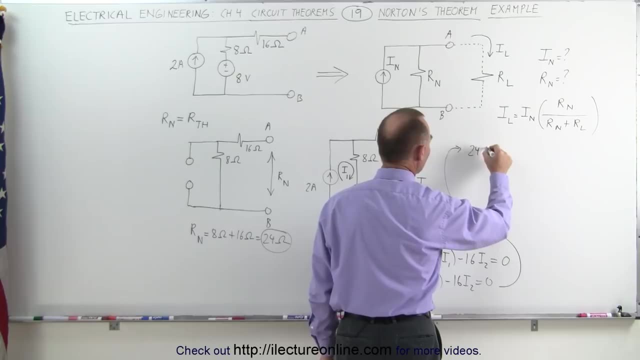 other side I have a minus 8,, minus 16, that's minus 24,. well, when I move to the other side, I get plus 24, so let me go up here. So we have on one side a positive 24. I2 equals. 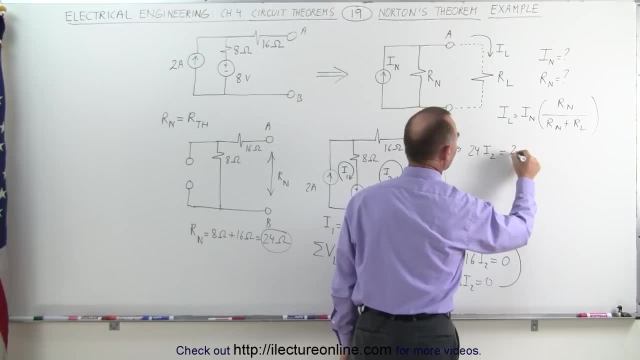 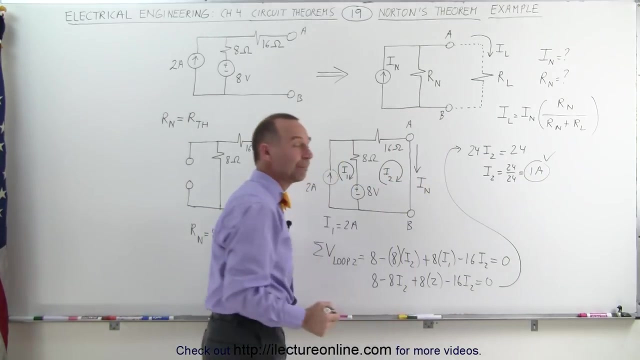 and on the other side we have 8 plus 16, which is 24,. therefore I2 equals 24 divided by 24, which is equal to 1 amp. So now we have Norton's resistance, which is, right here, 24 ohms, and Norton's current, which is 1 amp. I can now plug those. 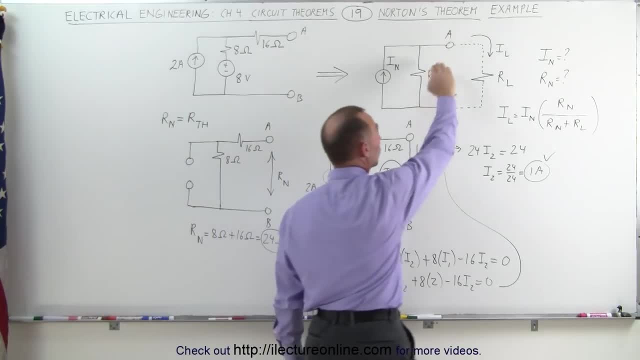 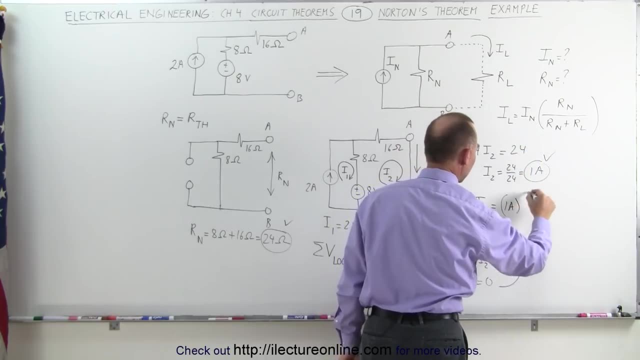 values into my original equation to calculate the current through my load resistor, I sub L. the current through the load is equal to I sub N, which is 1 amp times the ratio of R sub N, which we said was 24 ohms. 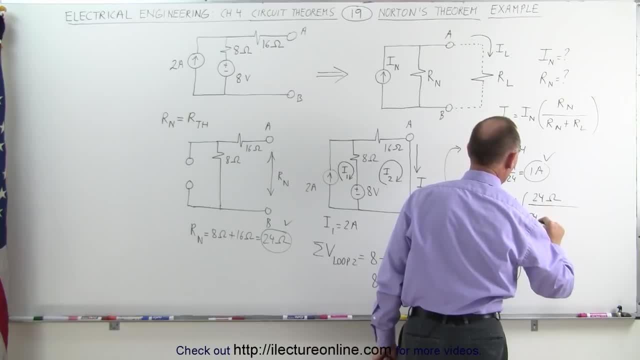 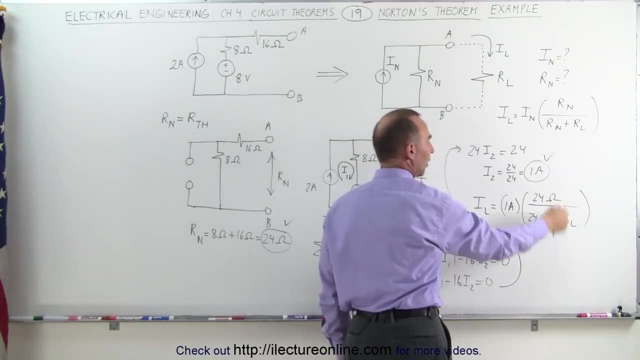 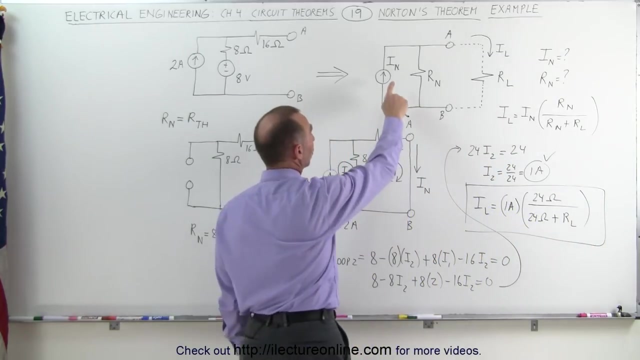 I2. I2. I2 divided by 24 ohms plus. whatever the load resistor is. All we have to do now is to find out what the current is through the load resistor by plugging in a particular value. But this is how we find the equivalent Norton circuit. We need to find the equivalent. 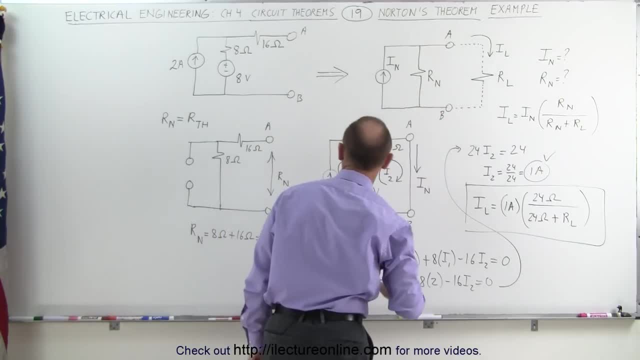 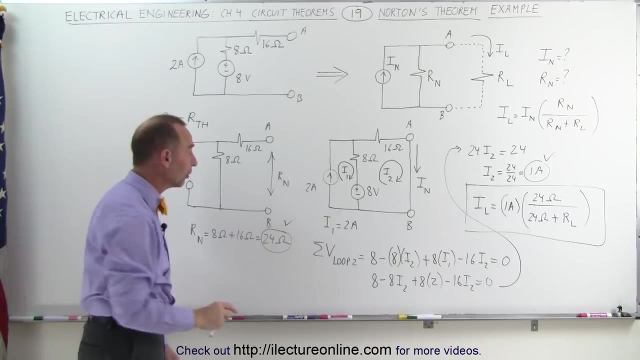 current and the equivalent resistance for the Norton circuit- Norton equivalent circuit. We find the equivalent resistance by removing any current sources and dropping any voltage sources to zero, And then find the resistance across the two terminals To find the Norton current. we're going to leave everything intact. 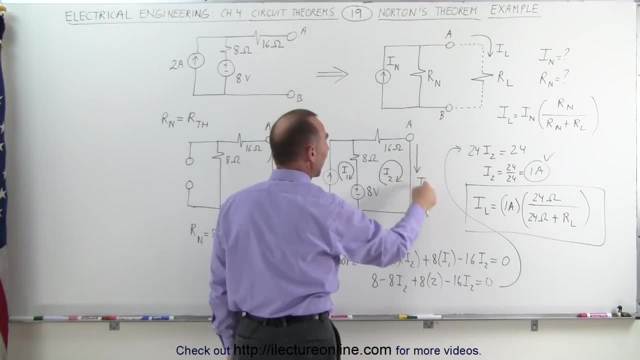 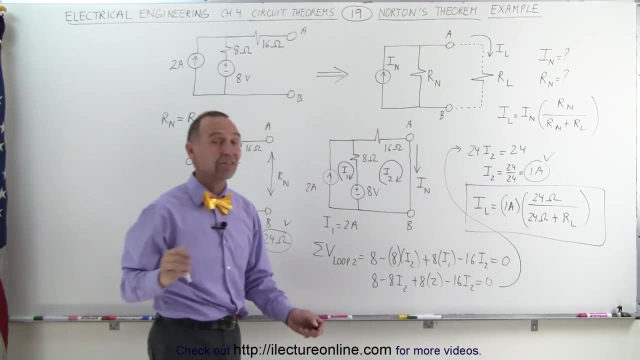 We're simply going to short out the terminals between A and B and figure out what the current is through that part of the circuit, through the short, and that will then be the Norton's current, And that's how we find the equivalent circuit. 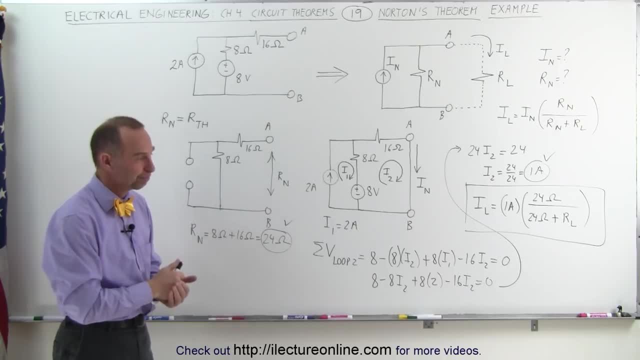 and that's how we find the current through the load resistor. That's how it's done. 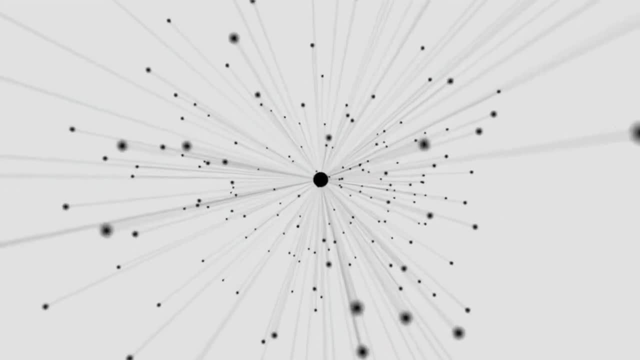 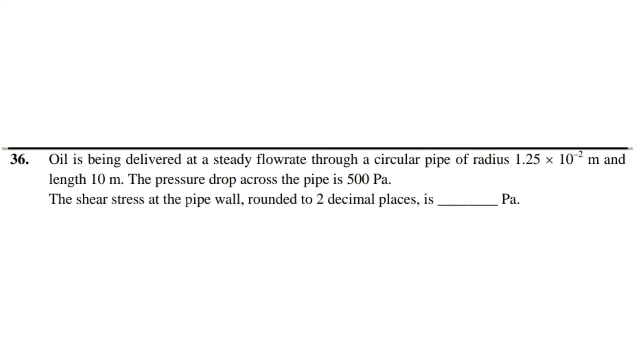 Hello gate aspirants. welcome to gate chemical solution channel. This is two more fluid mechanics question in the year 2017 gate question paper. Please read the question very carefully and identify what is given and what we have to find out. If you look at the question, it is mentioned.